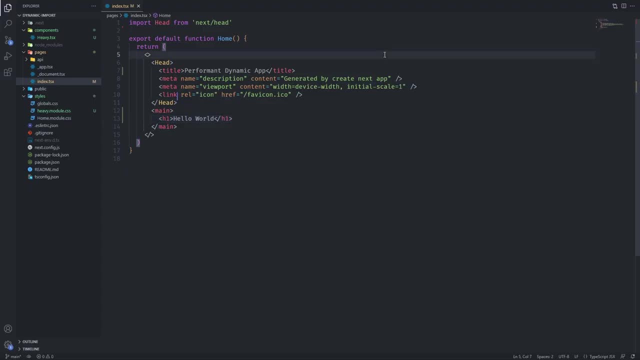 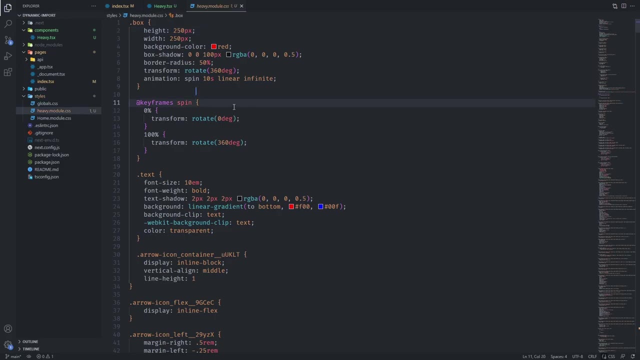 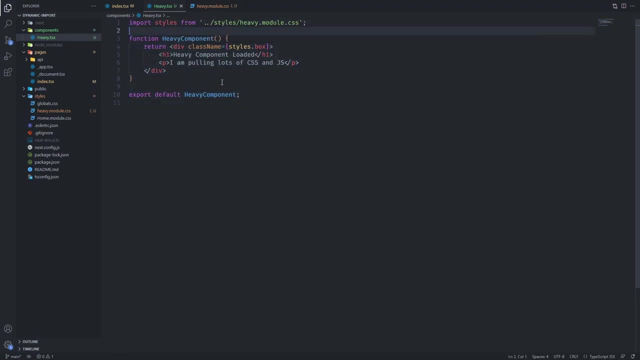 Which is not enough. Now let's say that we have this heavy component that I made. It's just a heavy component that has styles, and these styles are just styles that I copied from a random page online. Okay, so there's, There's lots of styles here. So imagine that you have this component that's full of JavaScript, like 350 lines of JavaScript with random hooks used, everything else in between and this huge CSS module, right? 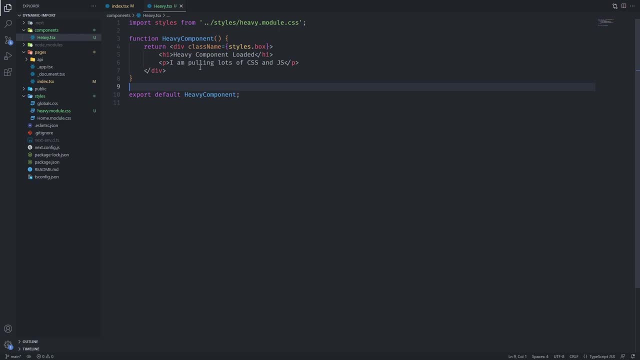 So this component is heavy and we don't just want to use this component and fetch it whenever we can, because this is going to be a strain on our network, right? Because we're going to pull lots of data. Now, What we want to do here is we want to show this heavy component only when the button is pressed. 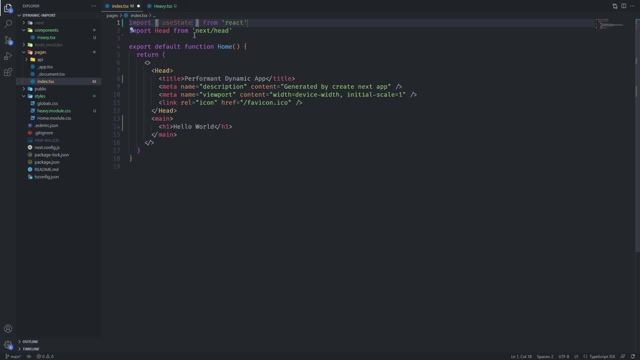 So let's implement that. That's the first step to show off the real power of dynamic imports. So let's just create, Get a useState hook, create a state. So we're going to say const should show and set should show, And it's going to be false at the beginning. 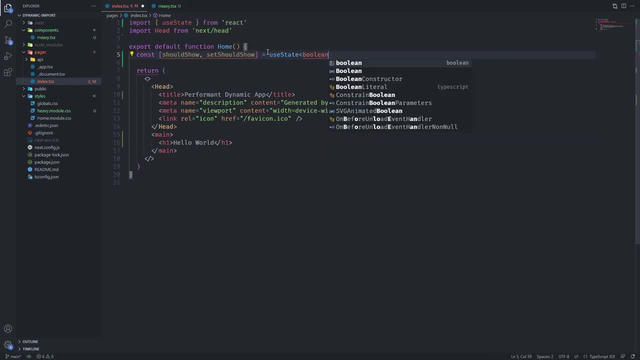 So we're going to say boolean, Not like that. Boolean, Okay, False. And we're going to have a button here And we'll say click me. And we're going to give it an event that says set should show to true. 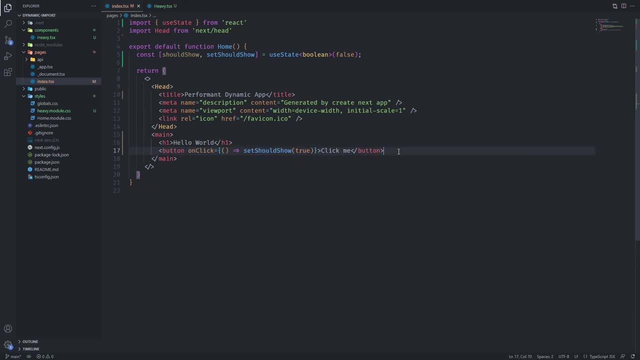 To true. Okay, Now we want, when this should show is true, we want to show the heavy component, right? So we're going to say if should show. and So this basically means, If this is true, then you're going to render, you're going to return what's after the end operator. 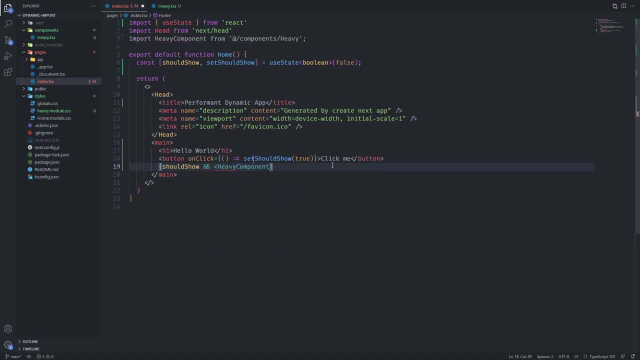 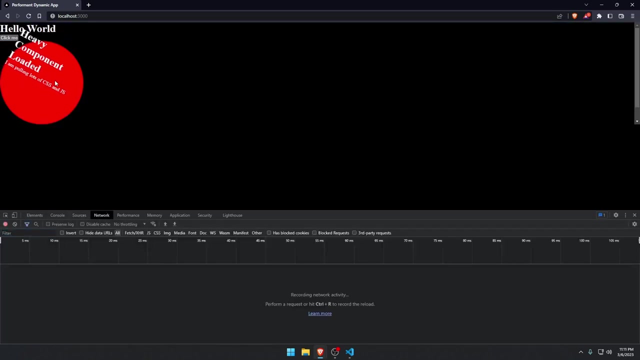 So we're going to return heavy component. Okay, Now it should work. So let's try it out. Now we can go to our page back. Okay, And let's go to the network tab. So this click me is working right. 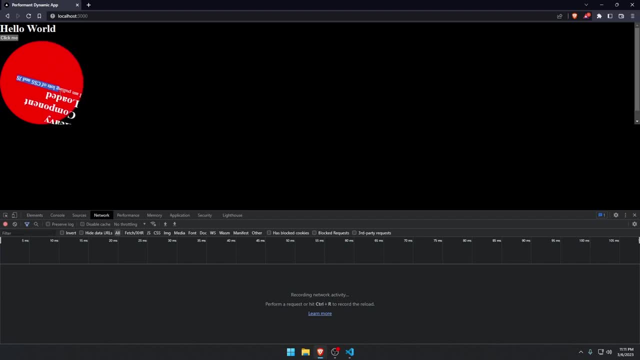 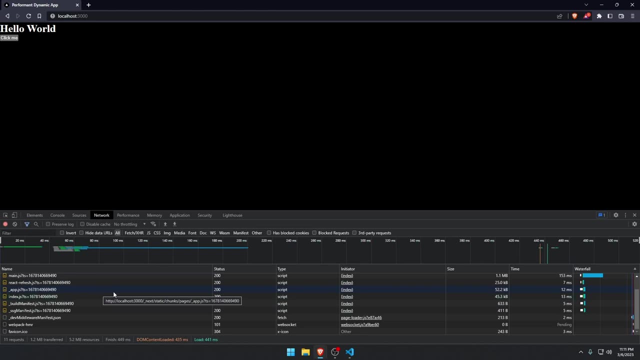 This is the heavy component that's loaded, And I'm using lots of CSS. Okay, That's what it says. Now, when we reload the page, we see that this indexjs, the same one from before, is now pulling 45.3 kilobytes. 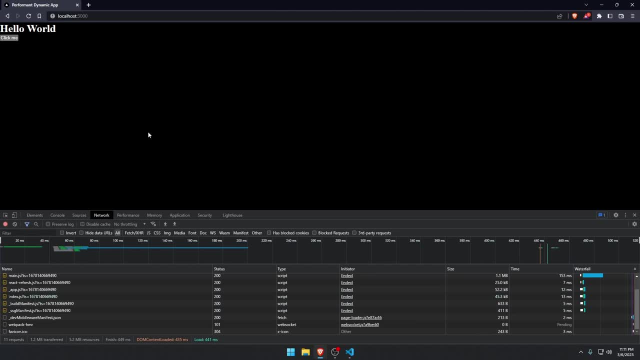 Now that makes sense right, Because we imported that component and we're using it, But at the same time it doesn't make sense because when we reload the page, we still aren't using that component. The component is not being shown. 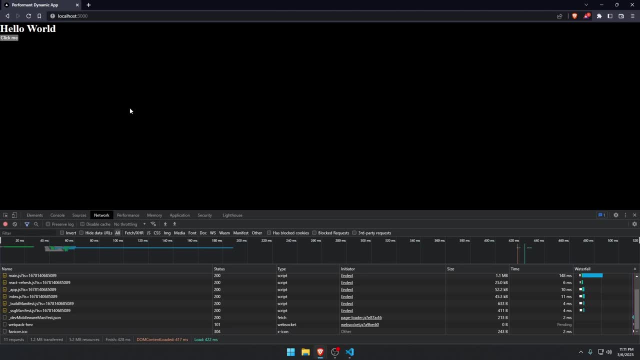 And who tells us that the user will click on the button and show the component right. So this component is potentially being pulled and not used, which means that here in our indexjs there's about 40 kilobytes of wasted JavaScript. 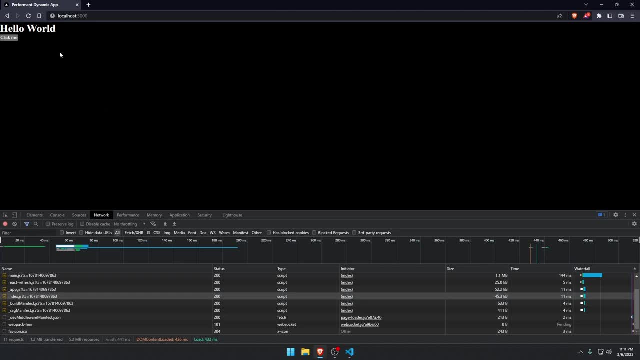 Now we want to only pull this component, the circle that's spinning with the text when, and only when, the user clicks the button, so that there is no extra JavaScript that's being fetched right. That's the important thing. So we want to use the next dynamic for this. 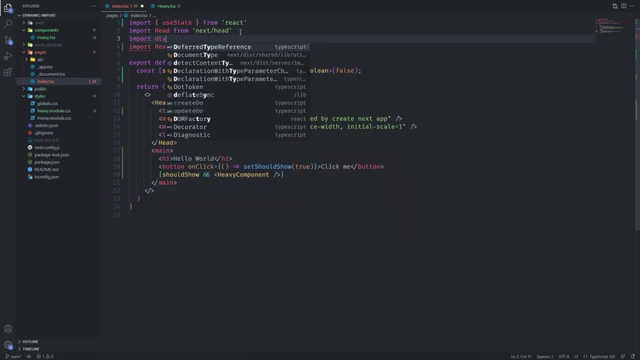 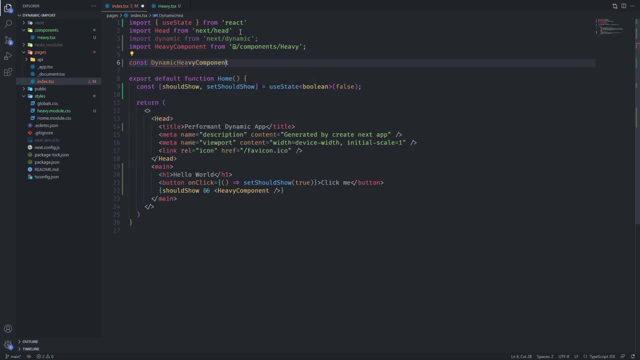 So we can import dynamic. next, dynamic, Let's say const, dynamic, heavy component. And we're going to say dynamic, We're going to give it a function that's going to import it. So we're going to go to components, go to heavy. 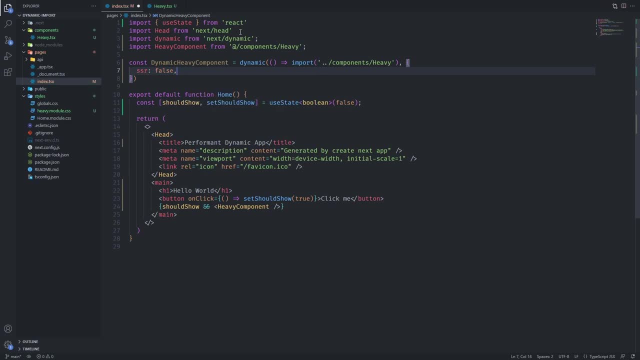 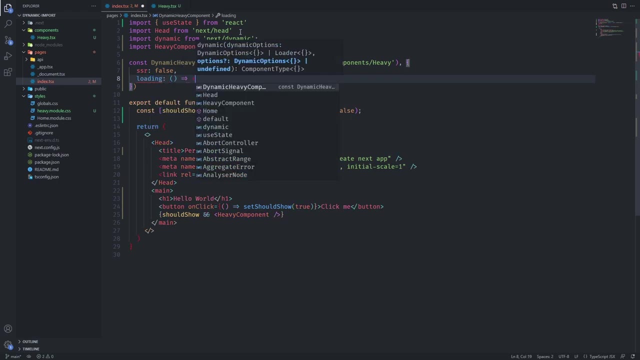 And we're going to say SSR is equal to false, because we want this to be fetched on client side And we want to say loading, And let's give it a function. Let's return, For example, AP tag And let's just say I'm fetching. 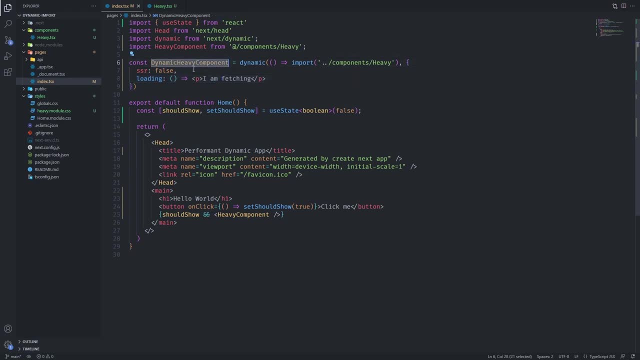 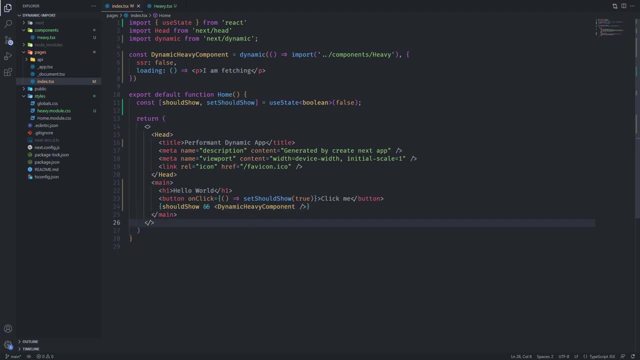 I am fetching. okay, Now this is the dynamic heavy component, right? We want to use it instead of the heavy component we imported at the top, So we can remove this component and use this one here. okay, And now when we go back to our browser, we reload the page. 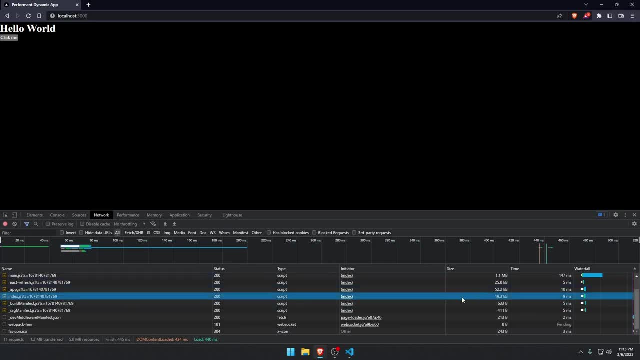 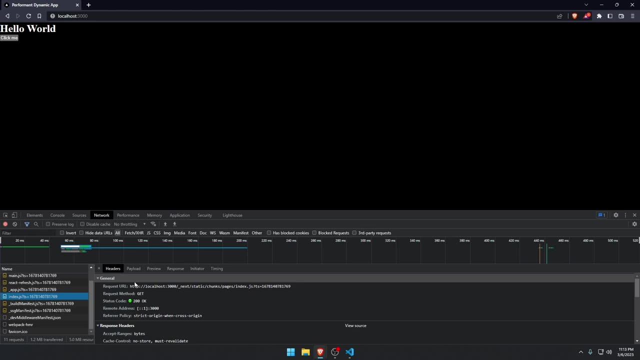 You can see that the indexjs is not. It's not the 55 or 45 kilobytes that it was, It's now 19.. It's way less than it should be, And it makes sense. Now watch when I click. 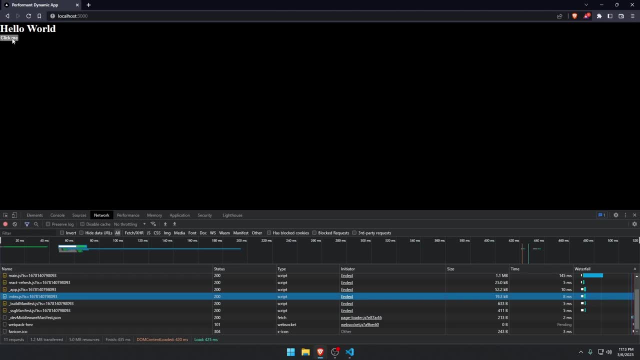 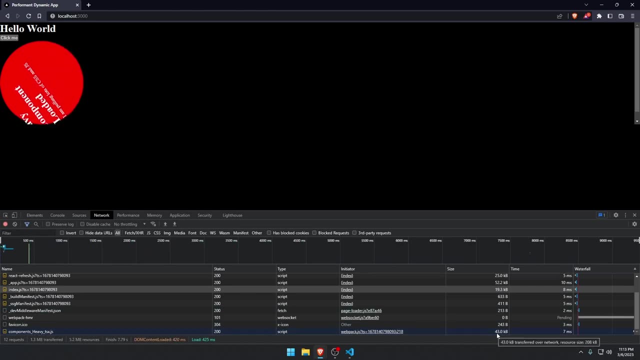 So 19 kilobytes. Watch when I click this button. Click it Now. you see the component heavy is being pulled. It's the entire 43 kilobytes of the component is only now being pulled, So not at the beginning. 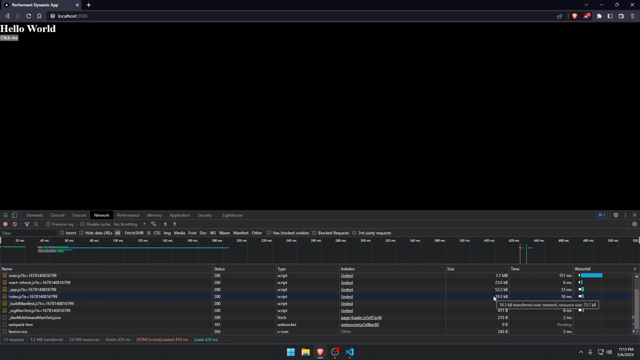 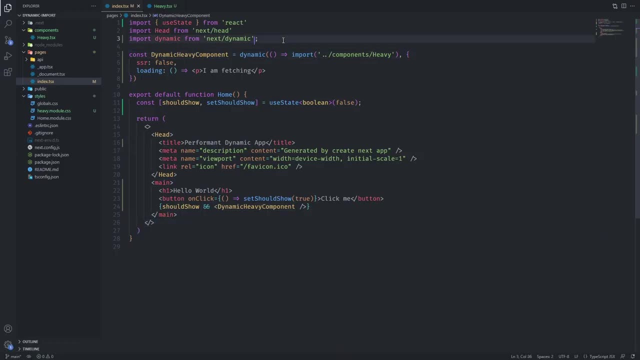 So we can. So we can, We can reload the page Again. indexjs. This is the first 5 kilobytes plus 15, I guess for the dynamic component The entire It's 19, because this is being imported. 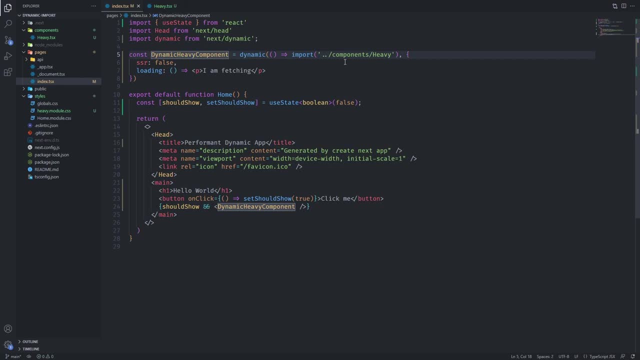 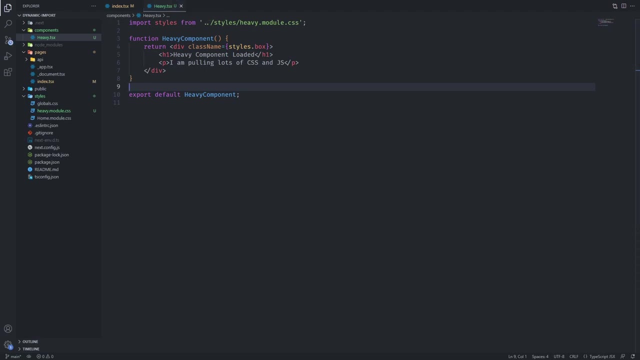 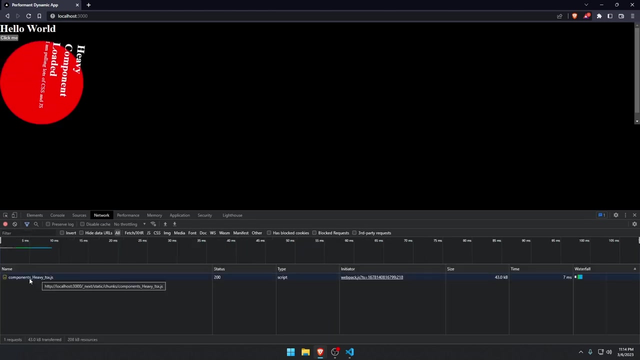 But now the entire component, this heavy component that we built out, that's pulling lots of CSS and JavaScript, is not being pulled. So it will only be pulled when I click the button And there it is. There it is The component heavytsx. 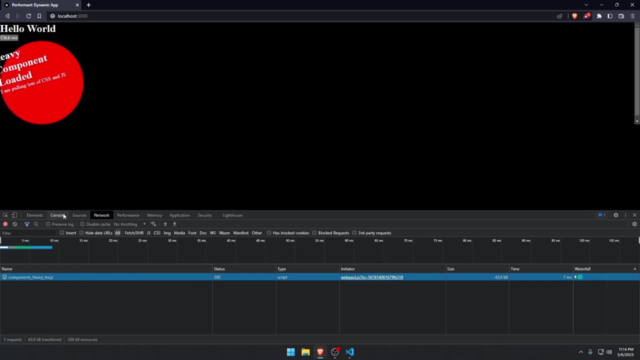 And right now we actually have a performant app that's not wasting any JavaScript. So we are 100% using the JavaScript. So you know, when you use the lighthouse feature here and it says there's unused CSS, unused JavaScript, unused stuff, like that. 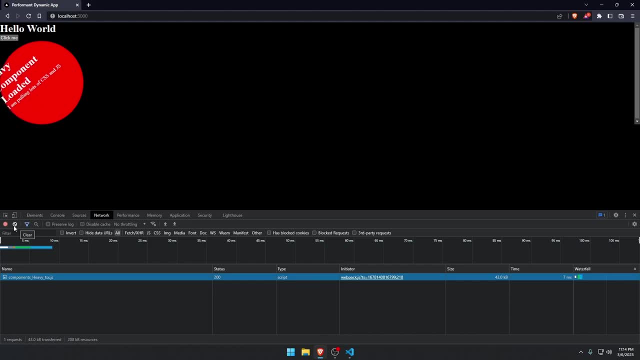 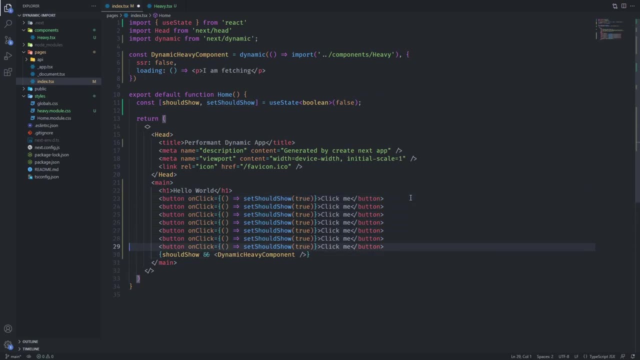 That's why, Because you're pulling JavaScript that's not being used. Because, let's say, we have, I have- 5 buttons here, Each of them that are showing something else. So let's say, click me 2,, click me 3,, 4,, 5,, 6,, 7.. 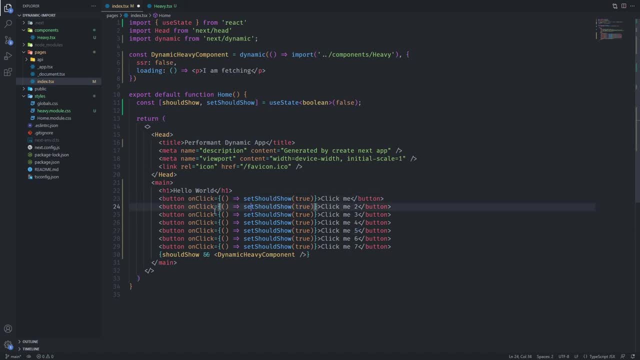 I know there's a shortcut for this. They can all show a different heavy component, right? The user maybe will click one button, maybe 2,, maybe 5,, maybe none, right? So imagine if there are 5 components like this: 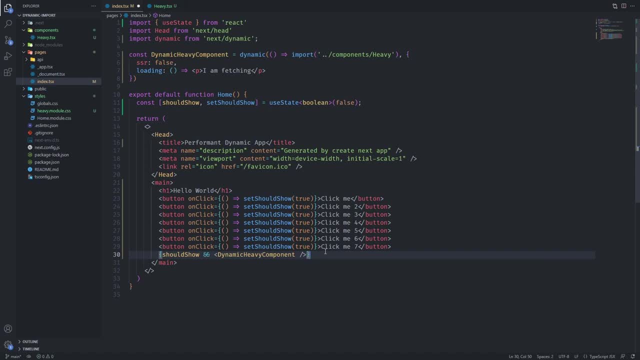 and they are all 50 kilobytes. That means that there's 250 kilobytes. That means 250 kilobytes of wasted internet. basically, You're wasting internet and you're slowing down the page. So this is when you want to use the dynamic import from Nextjs. 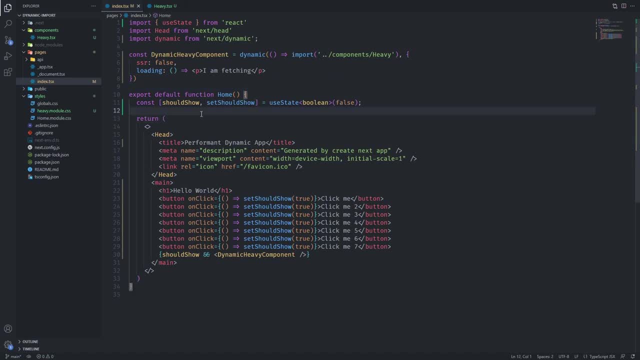 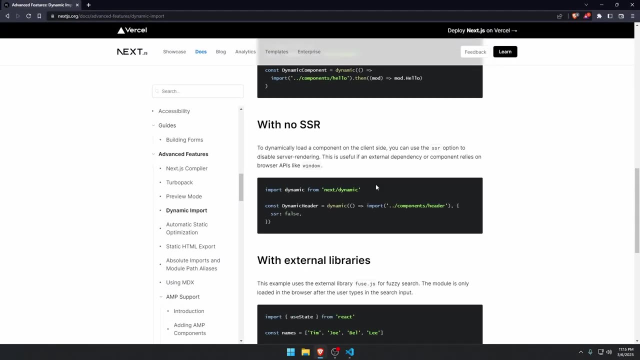 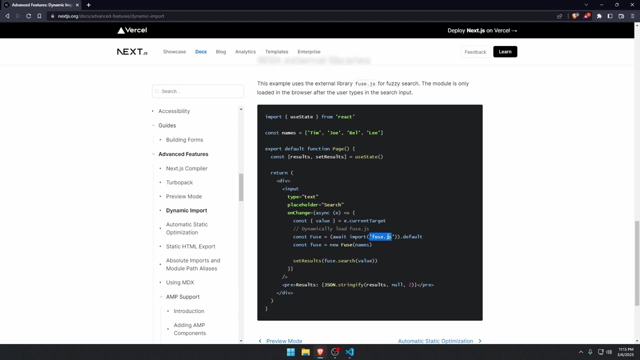 When you're loading something heavy and that you're not sure you're going to need it. This is a basic example. you can read up on the Nextjs site of more advanced users, for example. Okay, So you can see, there is an example where the FUSEjs 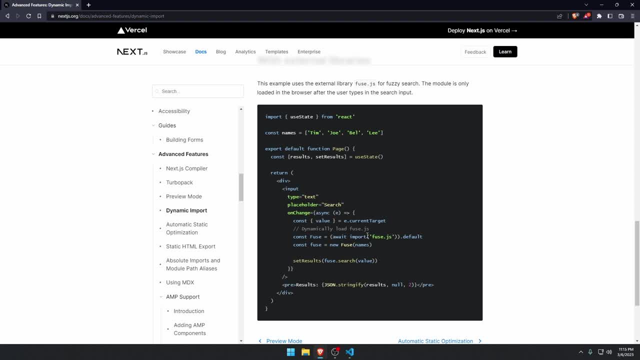 so the JS file is being imported only when it's needed. So, for example, it should be only imported when I click and search on something. There's no need for that JavaScript to come on my browser if I'm not going to use it.